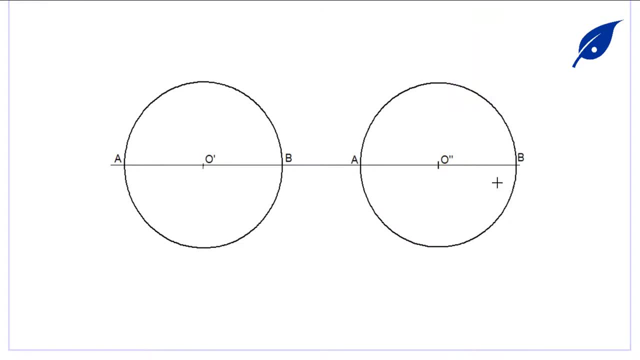 on the side where the horizontal line touches the circle. you mark A and B on both circles, that's with the center O' and O''. Then we draw a perpendicular line passing through the center of each of the circles, So in that way we can be able to get a given radius. 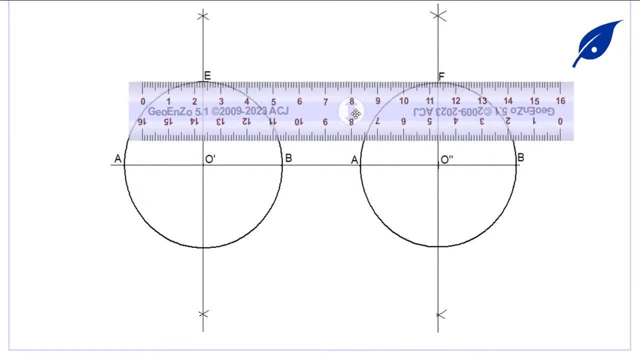 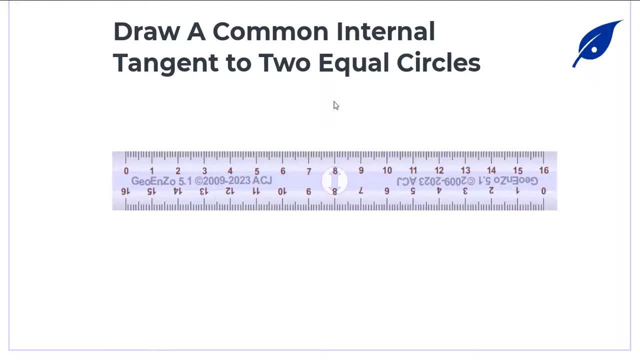 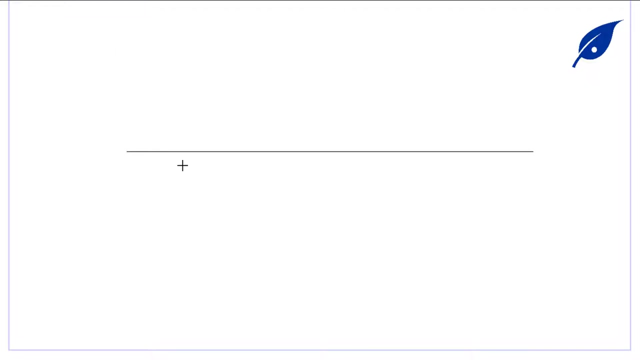 Where the edge of the circumference which will give us the tangent at the point E and F on both circles. In this video we shall consider the construction of common internal tangent of two equal circles. Now the first thing is to draw a horizontal line. On it. we mark the points A and B which will be the center of our circles. Now, at the point 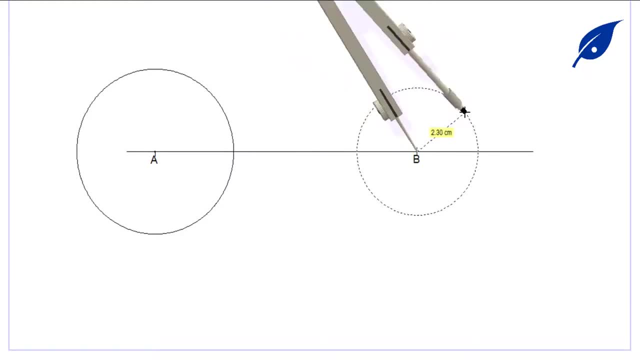 A, we draw our circle, then the distance between the centers of these two equal circles will be A- B. So at that point B, we draw our circle. Then now we bisect the line AB to give us the midpoint, Which will be C. So we connect the line at. 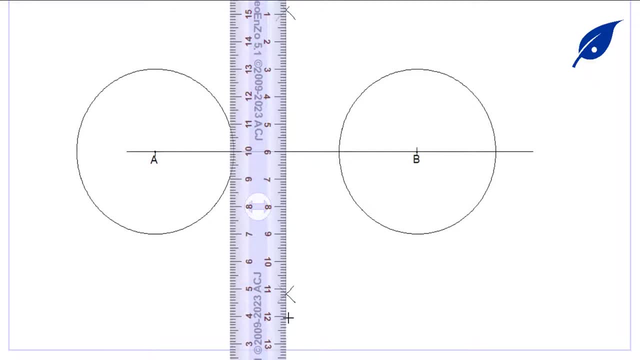 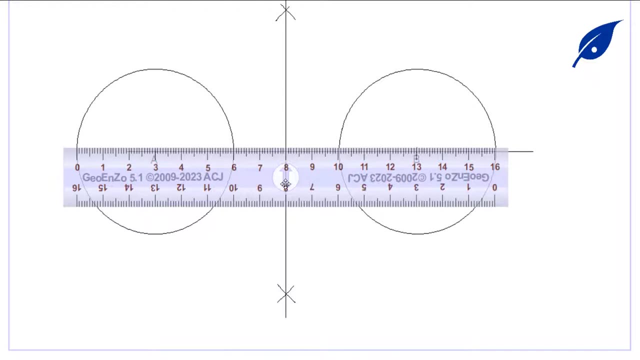 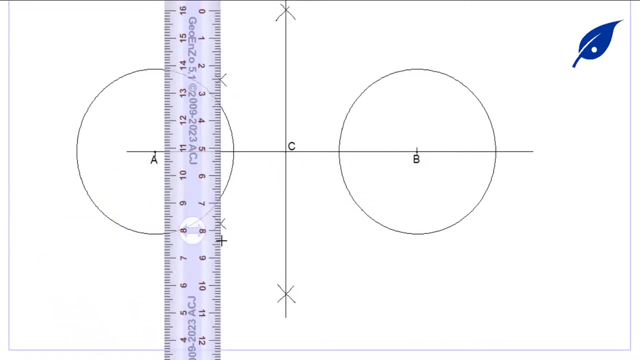 this point, Which will give us C. So after getting the point, see, now we bisect the line EC so that we'll be able to get a semi-circle which will help us in getting the point where it will be the tangent for that circle. To achieve this, we first have to draw the arc at the 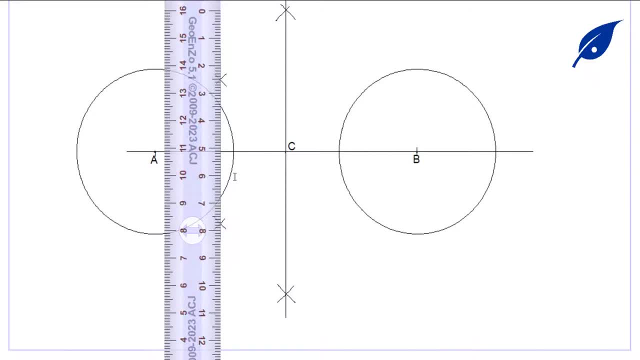 center where the line will go towards the middle and we see the predetermined acne points. This should be the the default slope that we are gentling to this curve. It should be very that will touch the circle with the center E. so at this point we draw a semicircle. so at the point 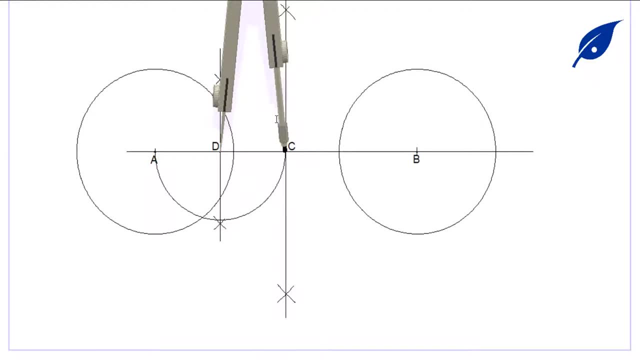 where the semicircle touches this circle with the center E, that will be the point where it will give us the tangent, which is the point E. so we connect a line from E passing through E. so with that line we produce a parallel line radiating from the center of the circle B, so the edge of this. 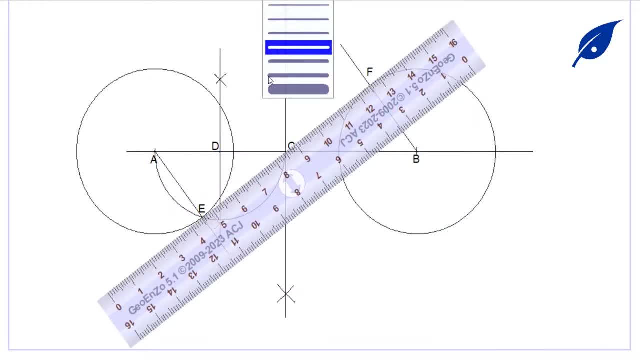 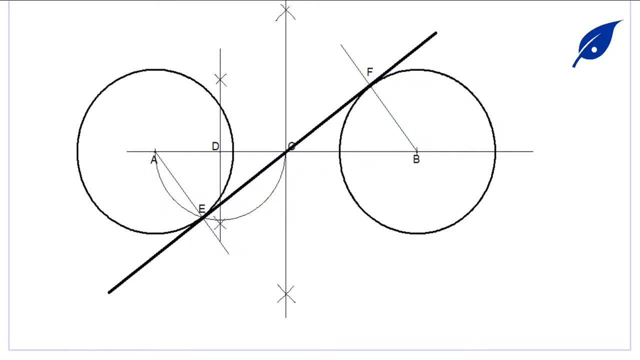 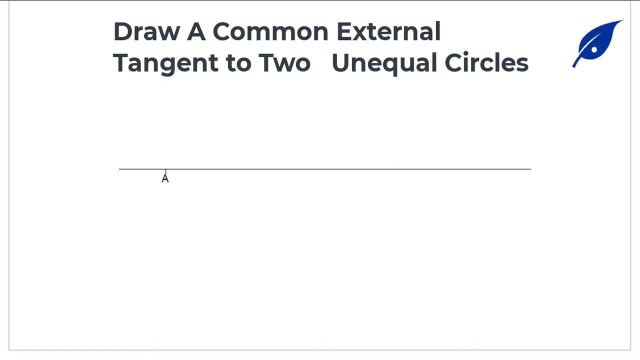 circumference of the circle where it touches will be F. so connect the point E and F to give us the required tangent. in this video we shall consider the construction of external tangent on two unequal circles. so the first thing is to draw a horizontal line against the center E and B. so 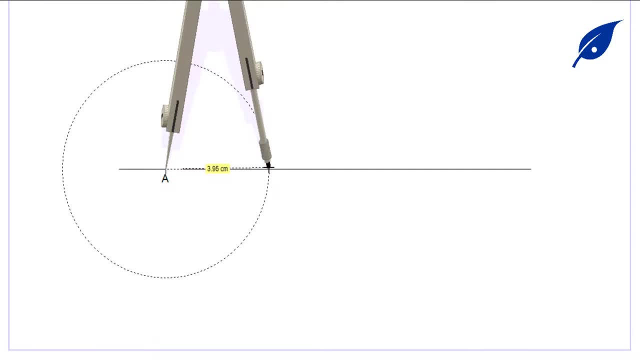 we will draw a horizontal line against the center E and B. so we will draw a horizontal line against the center E and B. so at the center E we will draw the first circle, which is the larger circle we draw at that point. then we will get the required distance between the two centers of the circles, which is AB. so at the point 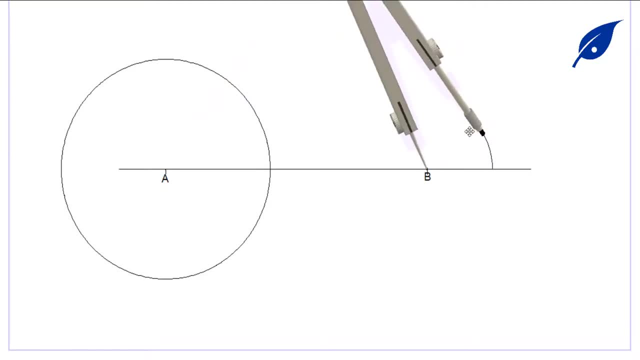 B, we will draw the smaller circle with the given radius, so after drawing it we will bisect the line and we will get the point. we now describe the position of the inner circle, which is what is known as a semicircle. then we mean by semicircle position here is Bn, and we will use the radius of the center at B for the distance we are drawing. 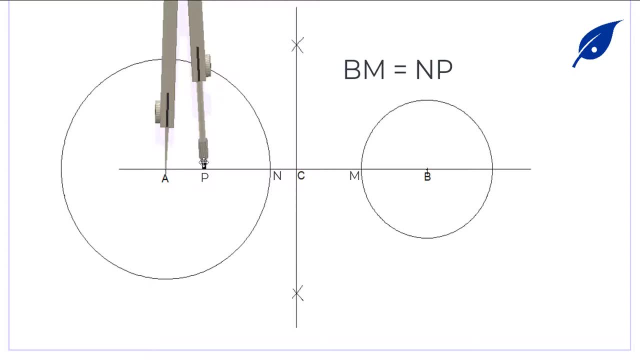 and we will draw a semi circle which isكN-4ab. we will use that ד-1ab, the的, we will get a semicircle which is BM and we will use that d-3ab to get the point NP. so BM is equal to NP. so after marking the point P, we draw a. 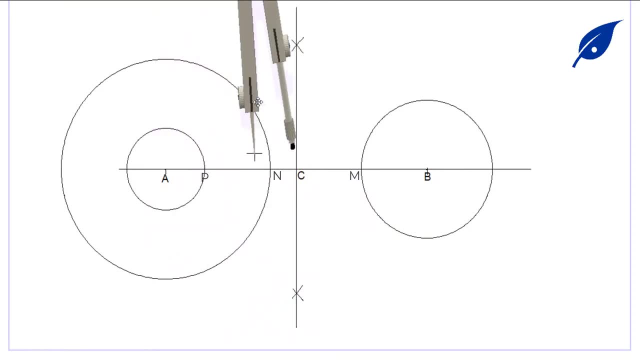 circle with the radius AP. the distance on the line AC will now mark so that it give us the circle which will touch the semicircle at a point D, then will extend the line AD to the line C, touch the circle at E. so with that we produce a parallel line on from the 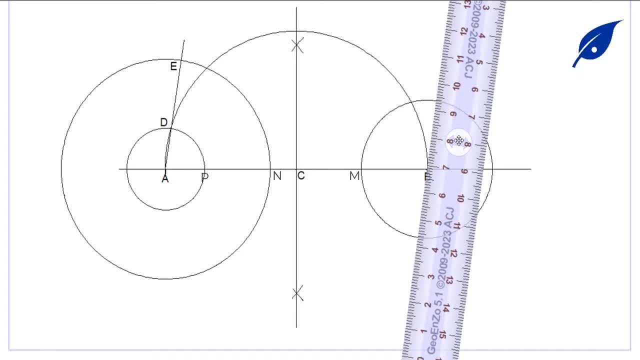 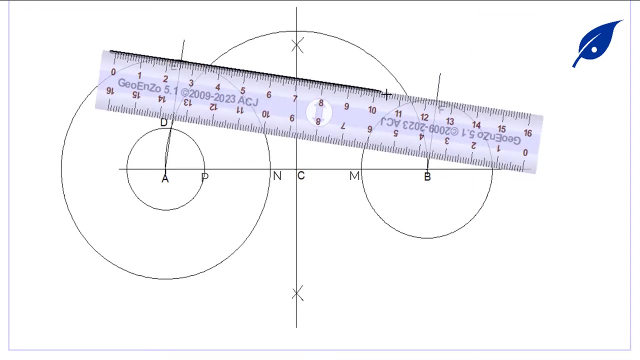 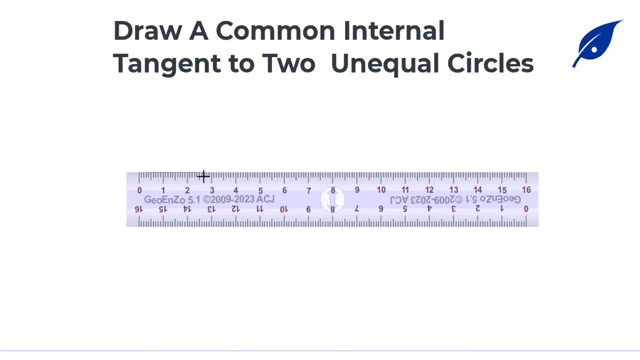 circle E on the circle B to give us the point F, so which will help us to get the tangent. so we connect the line from E through to F, which will give us the required tangent. on this one we'll draw common internal tangents of two unequal circles, so the 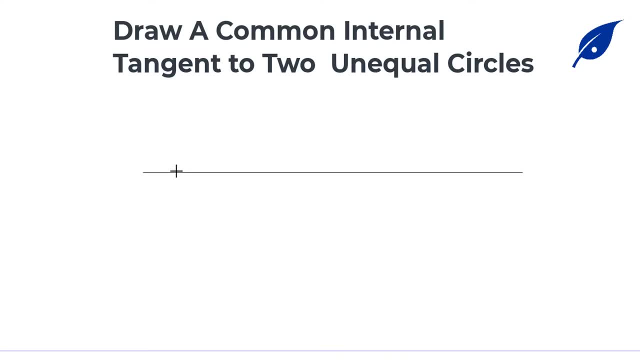 first thing is to draw the horizontal line and mark a point E. so after marking the point E, we'll draw the semicircle, the circle, at that point. then at B, we'll draw the smaller circle. now, the next thing is to bisect the line AB. so after bisecting the line AB, we'll get 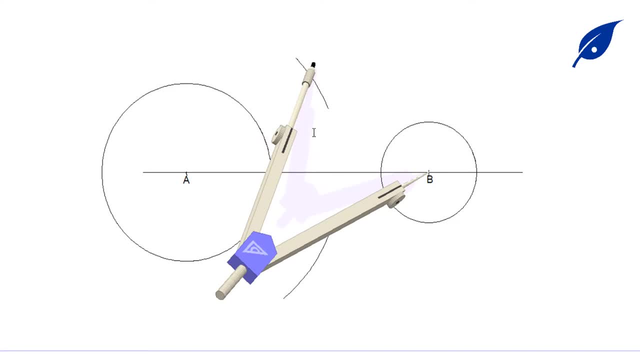 the new, the center, the midpoint, which is C. so after getting this midpoint, we'll draw a semicircle. we'll draw a semicircle at this point O, we'll draw a semicircle. so now the radius of our circle, smaller circle. we put it at the point D to get a distance outside the circle, because in 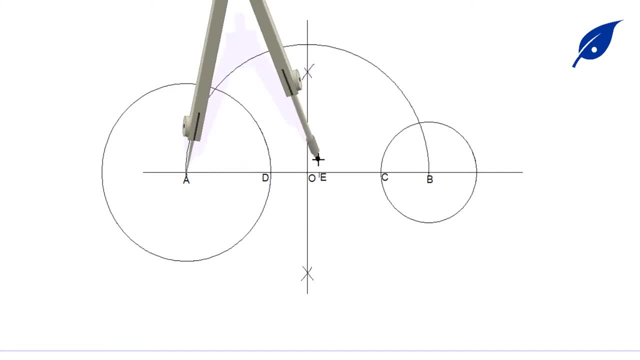 this one, we are constructing the internal tangent, so we'll get the point E. and now, with the radius AE, we'll describe an arc to minute this semicircle. at F we get a straight line from E to F, the line E f. we connect the line E F, so the line E- F will be parallel to a line coming out from the stable surface, that's F, and going to 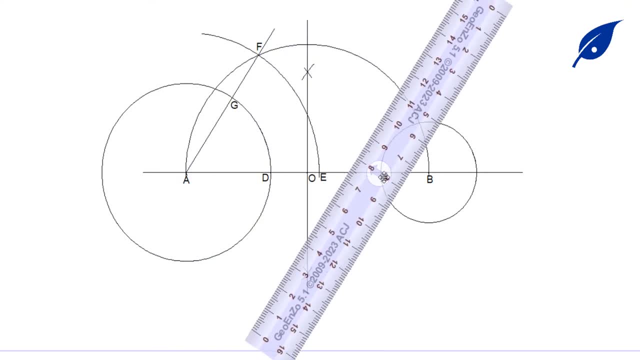 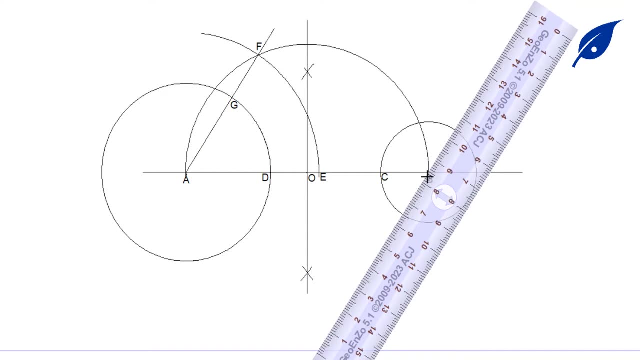 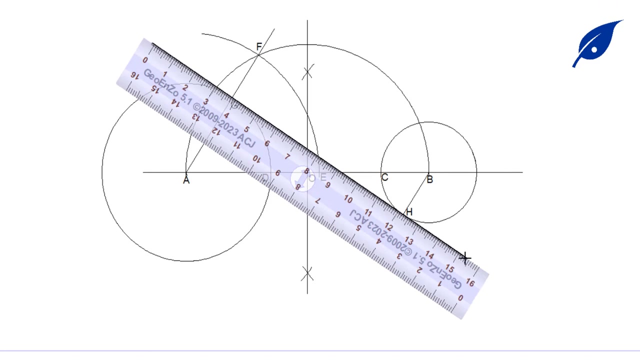 to F. the line AF will connect the line AF. so the line AF will be parallel to the line coming out from the center B. so the line coming will draw a line from the center B to give us H. so from H to G will connect the tangent, connect a line to give us the tangent. thank, 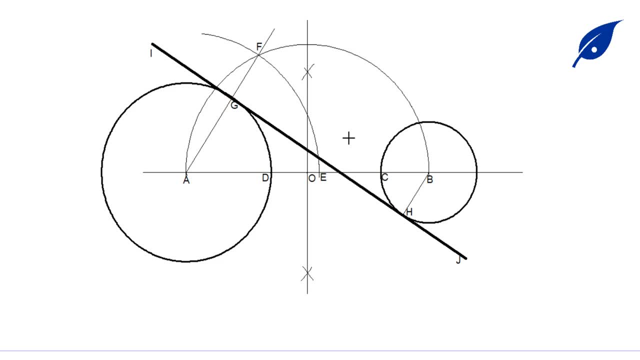 you for watching this video. make sure to subscribe to this channel for more videos.